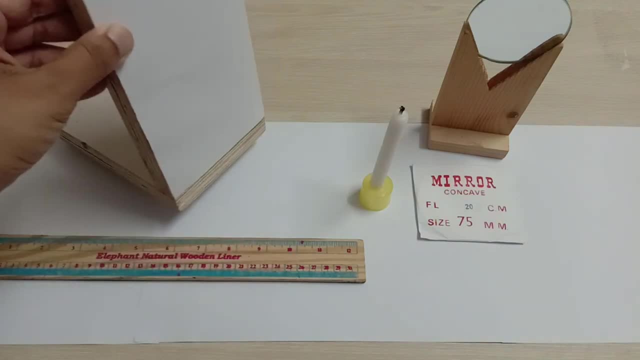 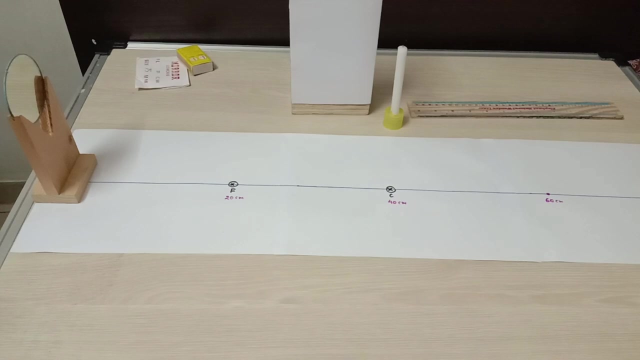 which I have fixed the A4 size paper, Because we are going to obtain the real images, and real images are obtained on the screen. So now let us move ahead with our experimental part. So here what I have done is I have joined three A4 size paper. Then I had drawn a line. 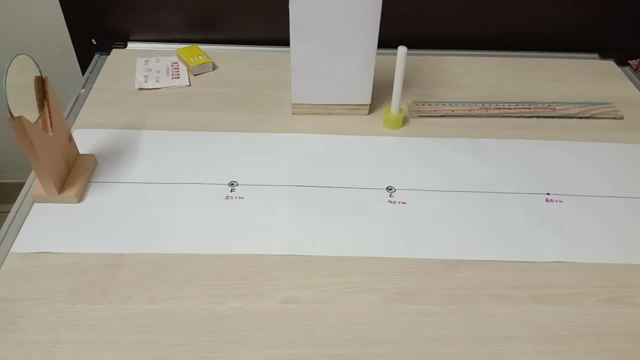 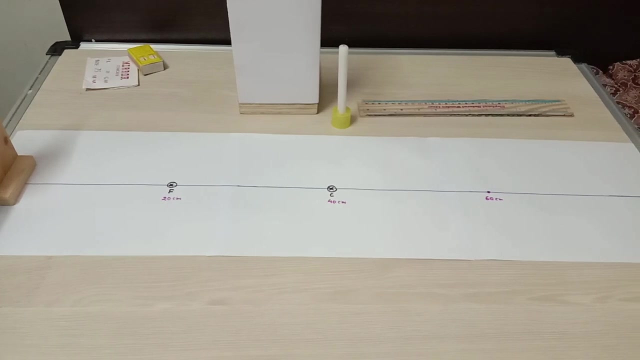 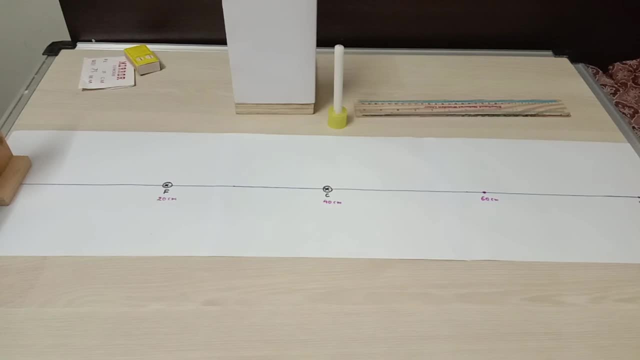 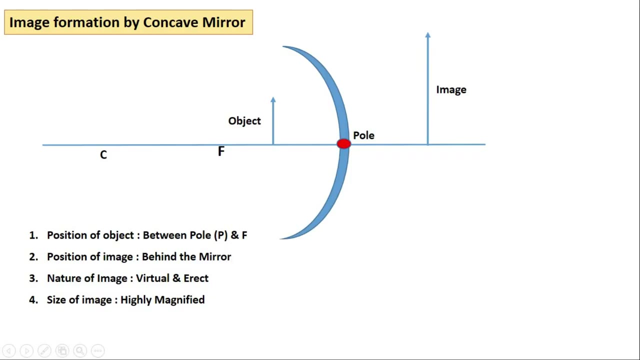 And we have done this to the surface, to the nose, to the face, to the touch, to the teeth, to the eyebrows, to the face and to the eyes. And here we are, And we are finished, We finished, We finished. 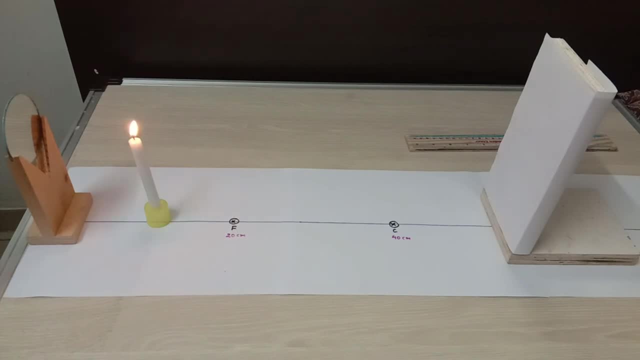 And we are going to do our two last steps. There we are. so, guys. the first case: the object is placed between the pole of the mirror and the focus. in this situation, we know that the image is going to be formed behind the mirror. it will be virtual, erect, and it will not be obtained on the 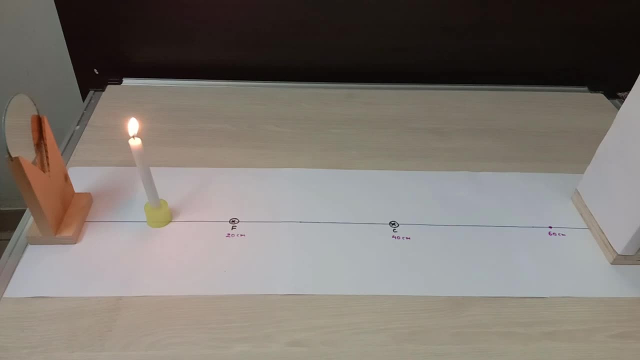 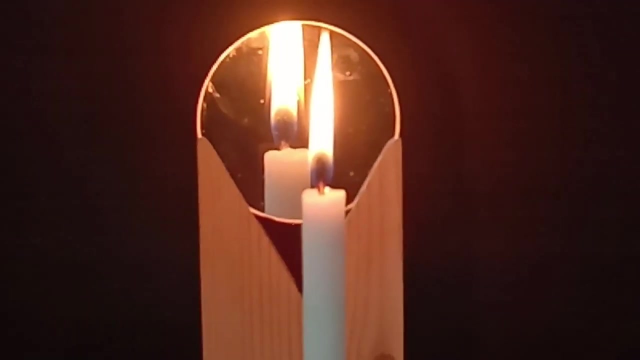 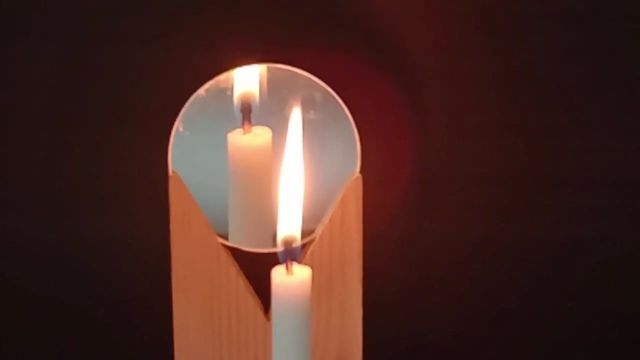 screen. so even if I move the screen backward and forward, the image is not obtained on the screen. now here, guys, you can see that on taking a closer look you can see the image is behind the mirror and the image is actually bigger than the object you can. 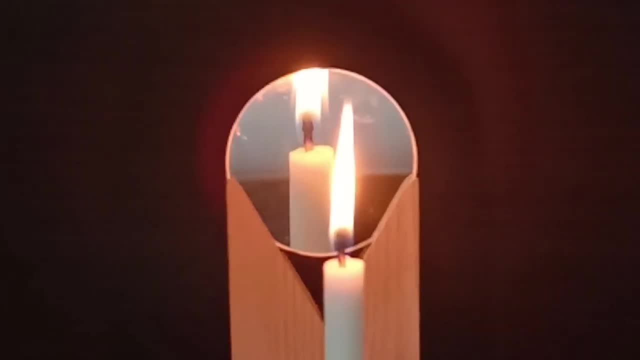 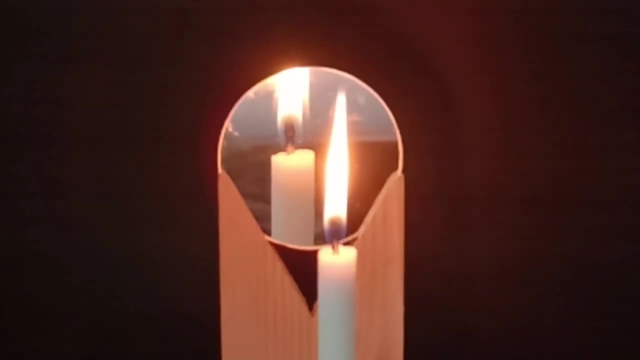 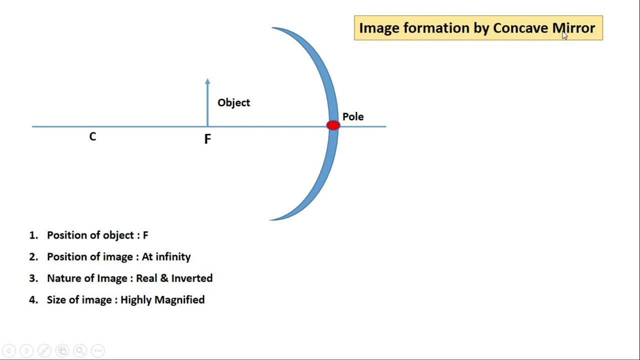 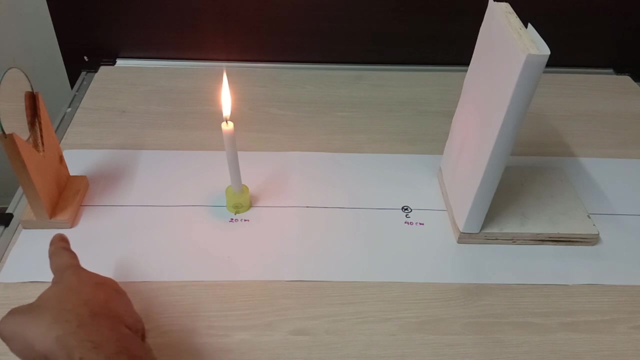 see the size of the candle being enlarged over there. now, the object is kept on the focus at a distance of 20 centimeters from the mirror. now, since the image will be formed at the distance of 20 centimeters. now, since the image will be formed at the distance of 20 centimeters from the 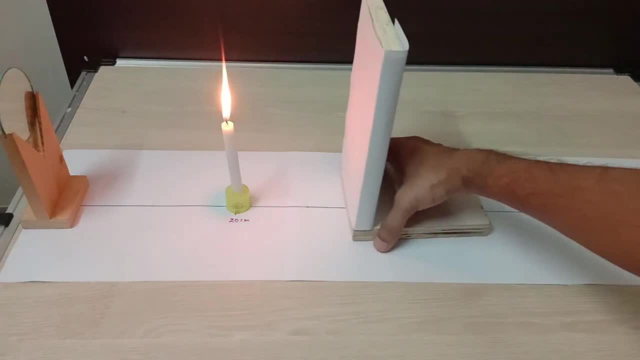 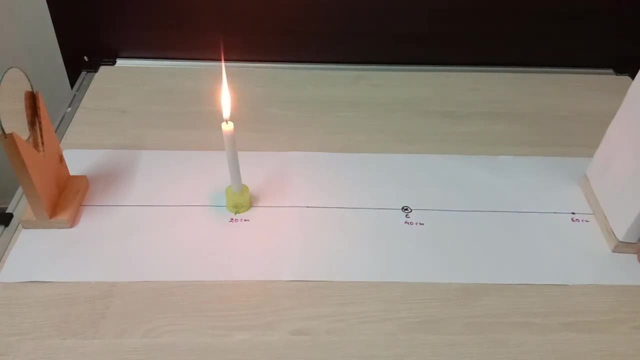 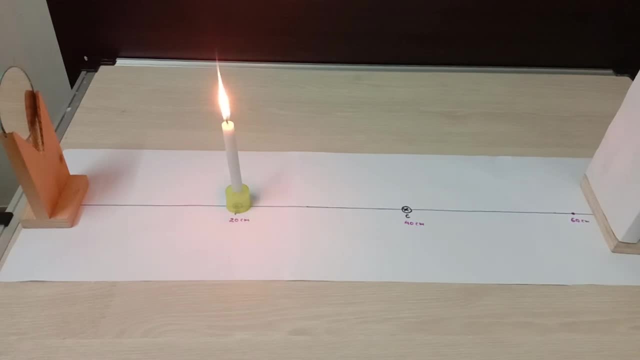 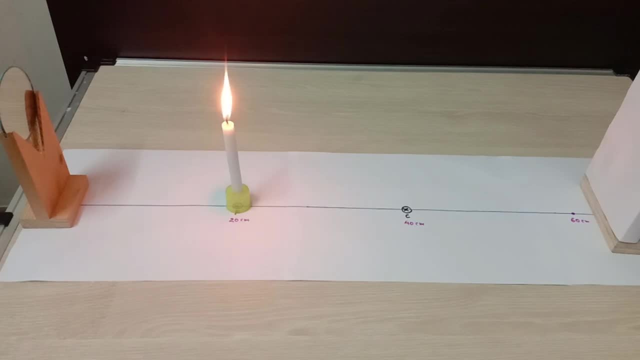 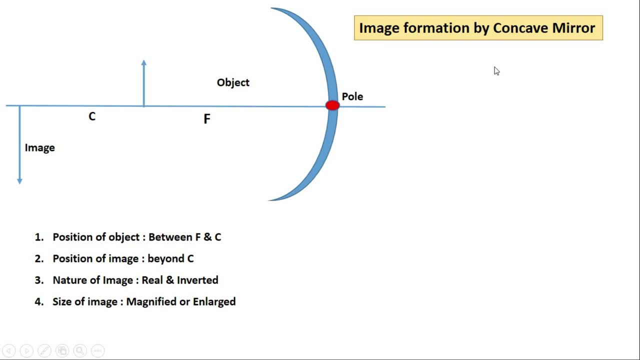 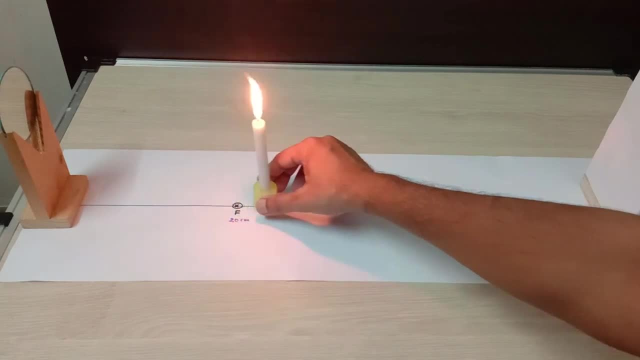 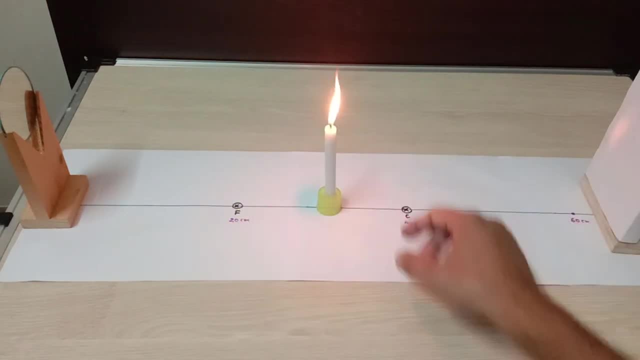 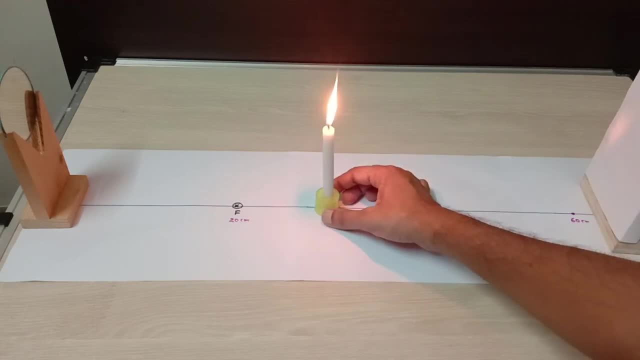 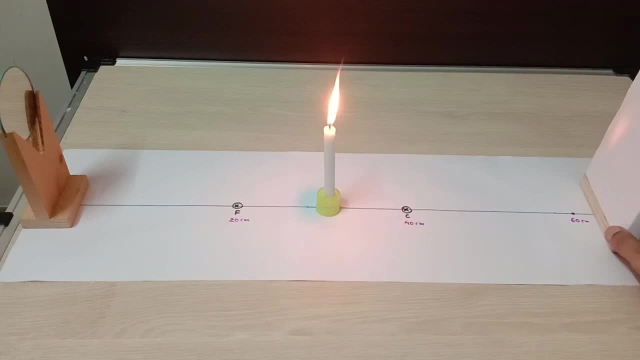 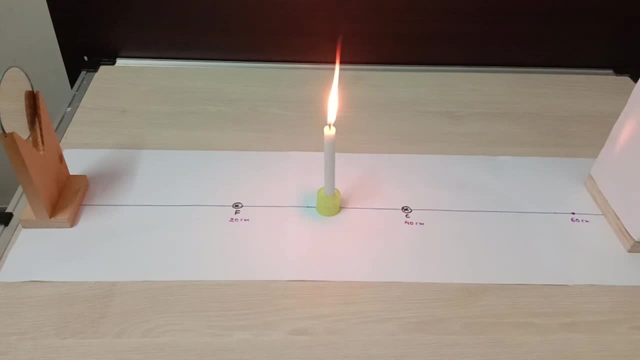 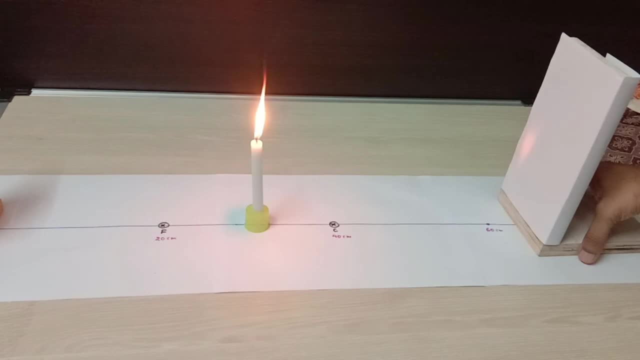 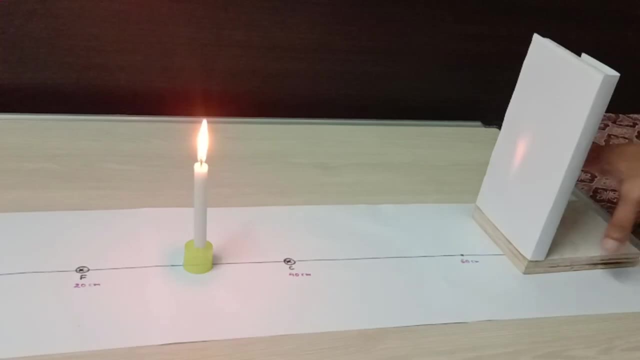 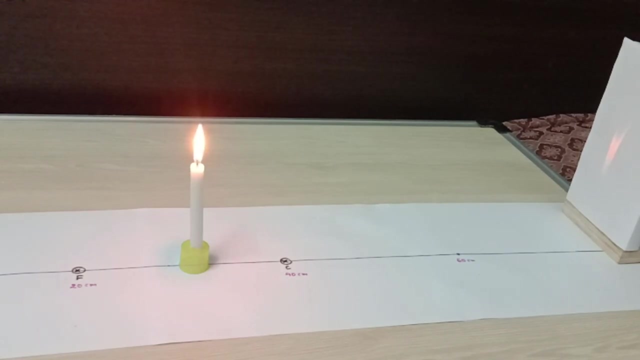 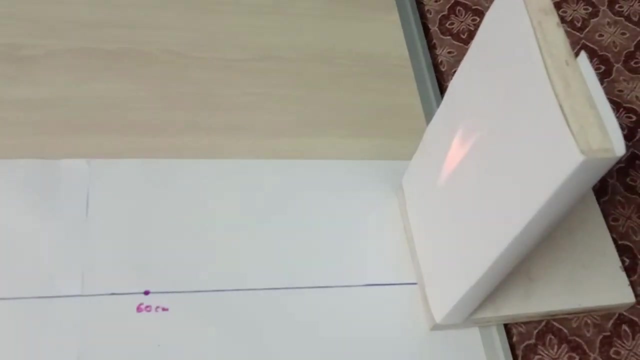 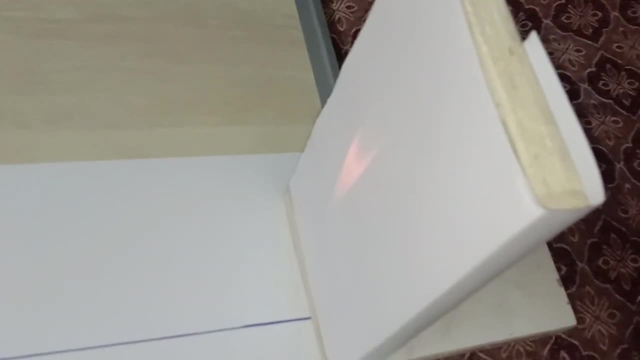 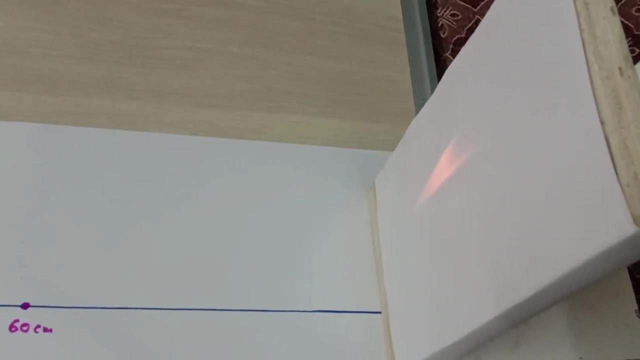 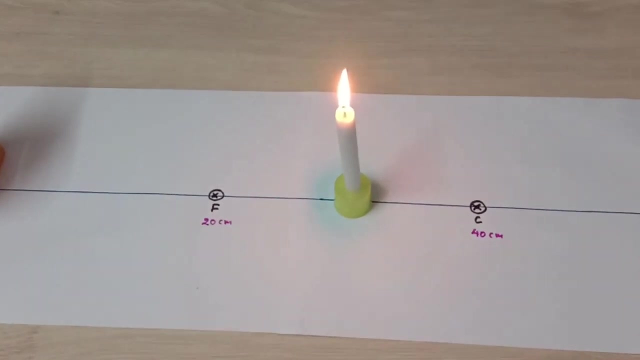 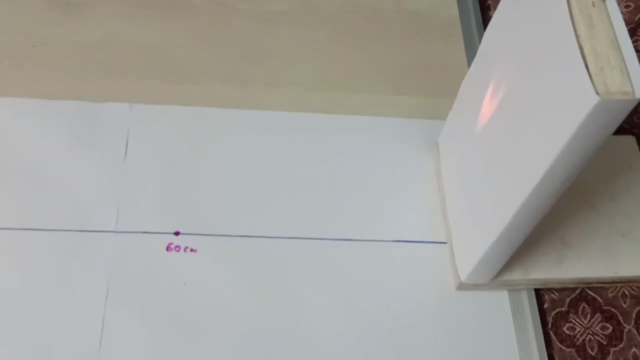 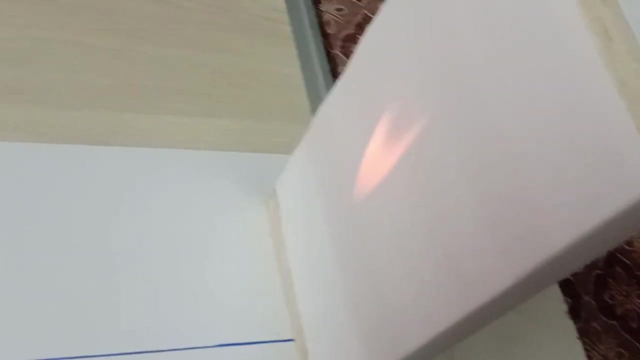 So the sharpest point would be considered as your image distance. You can move the screen forward and backward to check the sharpness. Wherever you get the sharpest image, that location would be your final image location. You can move the screen forward and backward to check the sharpness. 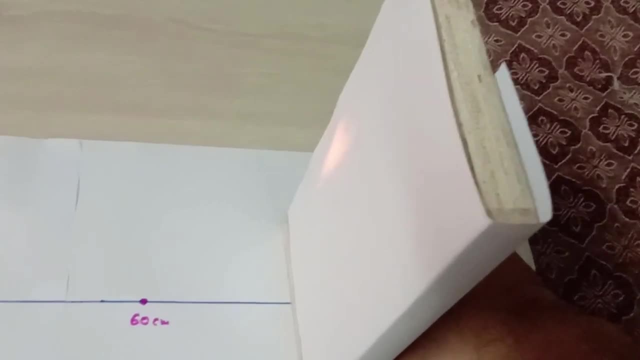 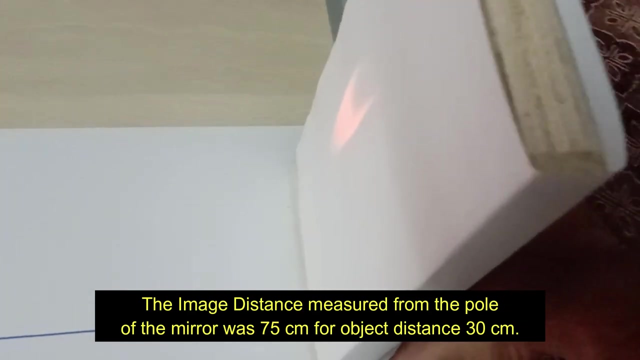 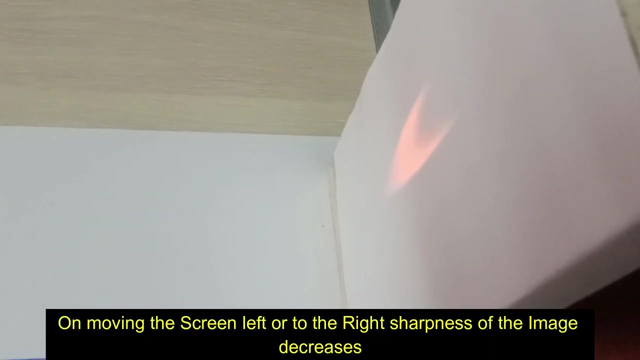 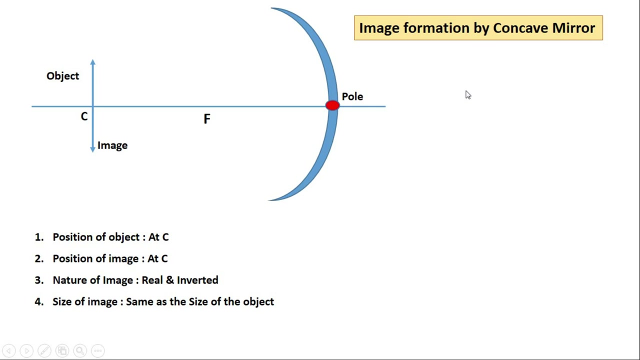 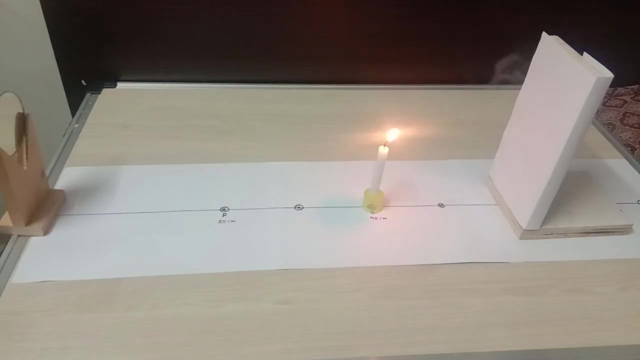 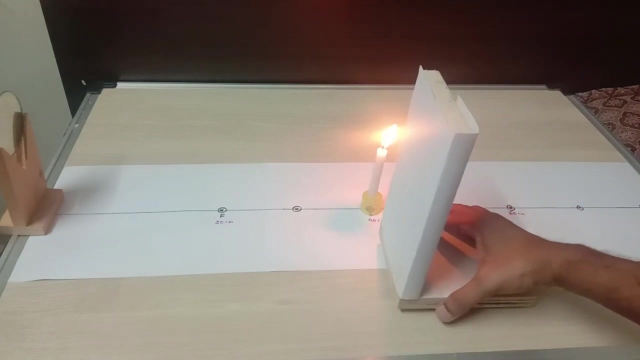 You can move the screen forward and backward to check the sharpness. Now the object is kept at C, So the image must be formed at C, Same size as that of the object. It should be real and inverted. Move the screen and hold the arrow at the center of the object. 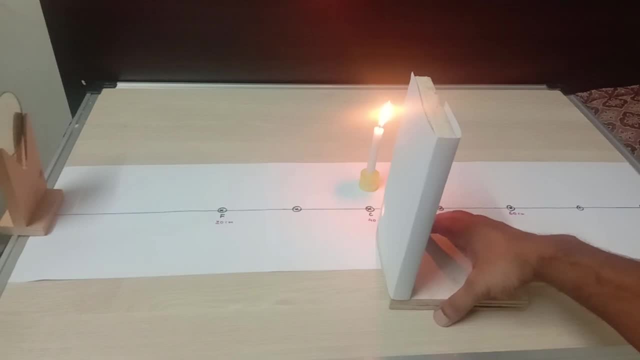 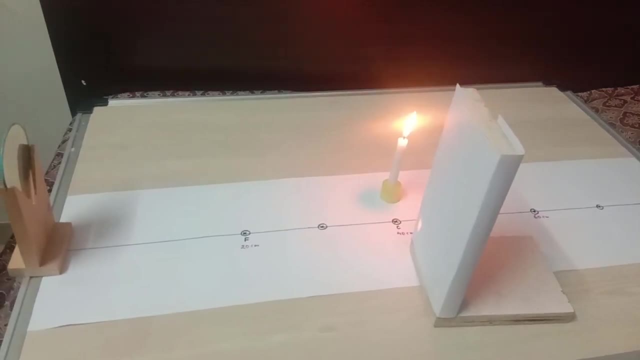 You can move a few inches of the object And select the shape you would like to select. The second option is to change the name of the object. In other words, the position of the object is important. You can change the name of the object as well.